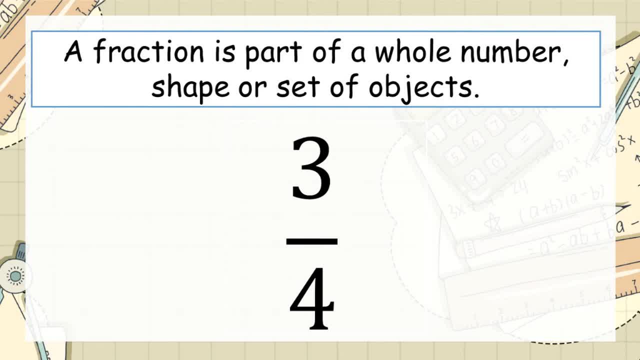 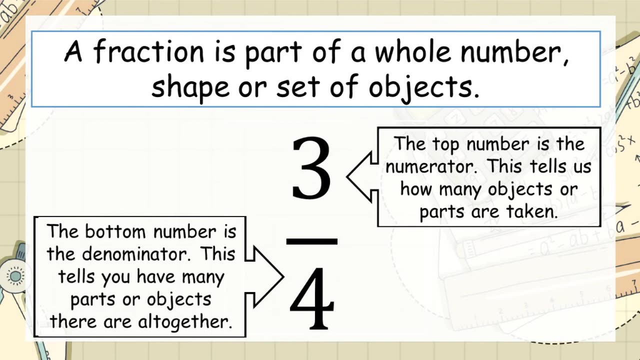 see if you can remember. Well, you might remember that the top number in a fraction is called the numerator. This tells us how many objects or parts have been taken. The bottom number is called the denominator. This tells us how many parts or objects there are. 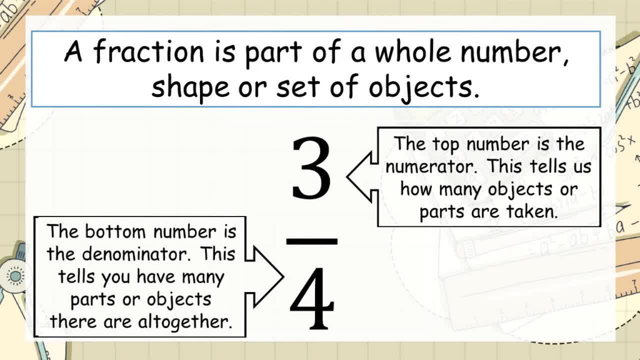 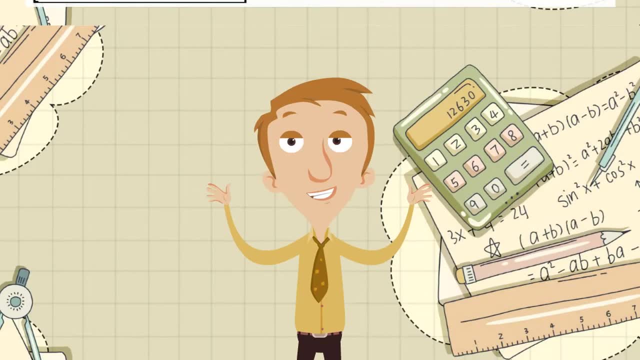 If you need a little bit of help remembering which one is the numerator and which one is the denominator, remember that the denominator is down under the line D for denominator, D for down. Remember that when we are finding fractions of numbers or sets or shapes. 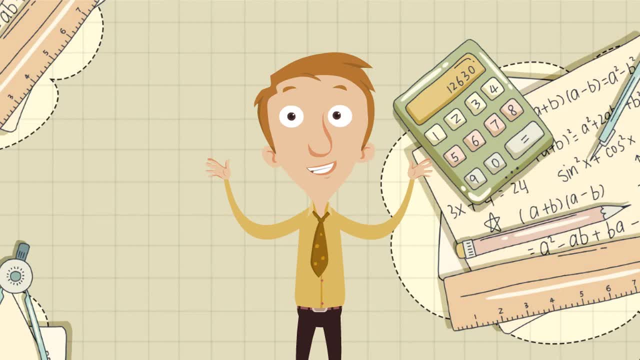 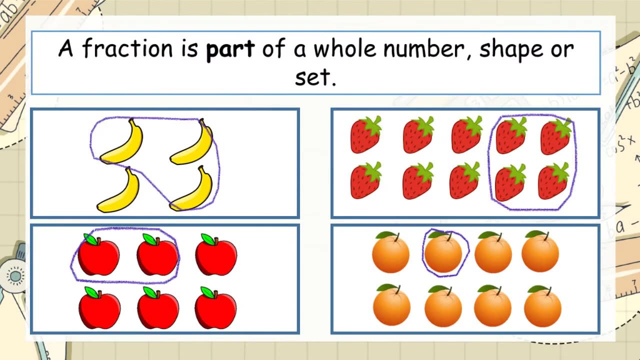 what we're really doing is dividing the number or the set into equal groups. Take a look at the sets of fruit down below. I have drawn a circle around a fraction of each set. Can you figure out what fraction of each fruit I have circled? Pause the video and write down the. 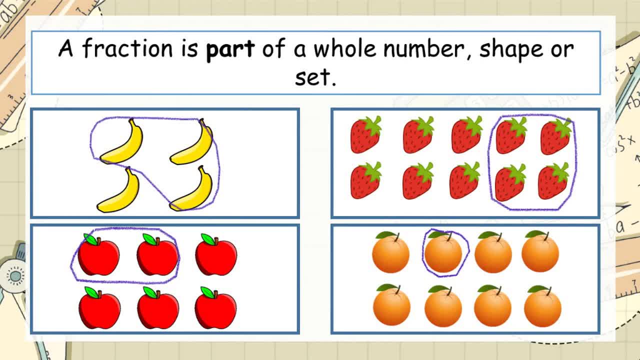 fraction of each set. Well, remember to figure out the fraction of the set. we count how many are circled. So we have three fractions. We then add them to what we call the numerator. What we have here is the denominator. So this is what we have. So this is our denominator. 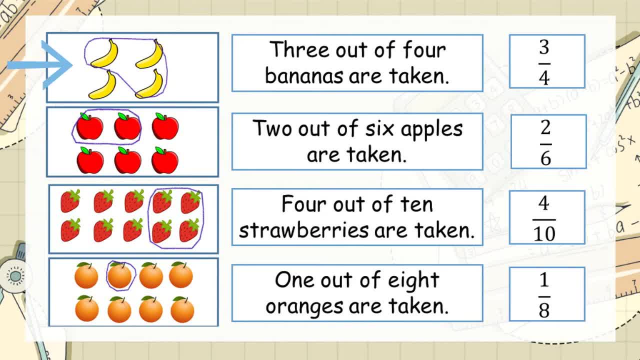 and this is what we get. That becomes the denominator. The denominator is one. So for bananas, that's going to be three bananas, That's going to be our numerator, our top number, And then we count how many there are in total. 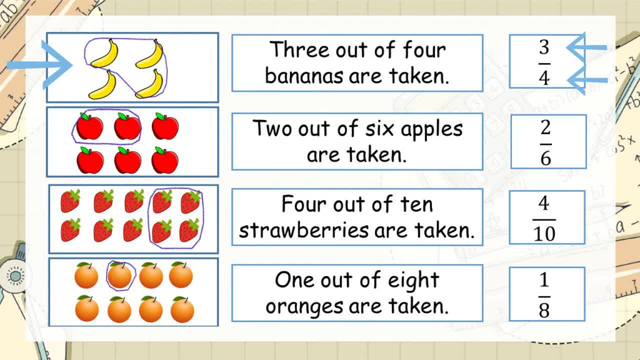 For the bananas there was four, So our denominator is four. We have taken three out of four bananas, which is equal to three quarters. as a fraction For the apples, we have taken two out of six apples, So that will be two-sixths. 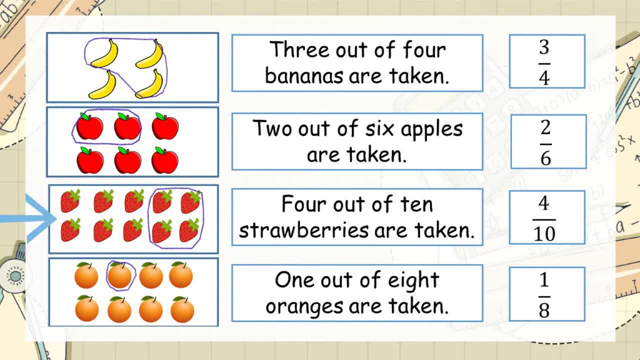 Which we write like this For our strawberries. you can see four out of ten strawberries have been taken, So that is four-tenths. We write that as a fraction like this: And finally, one out of eight oranges are circled. 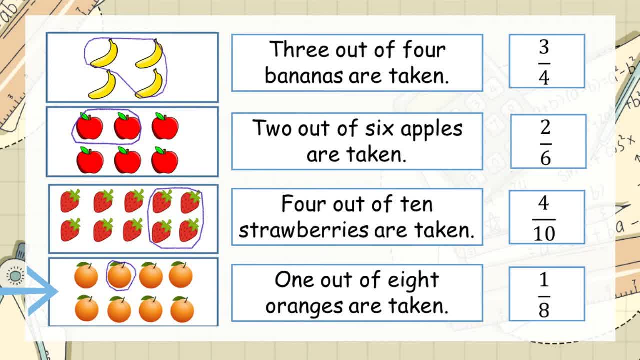 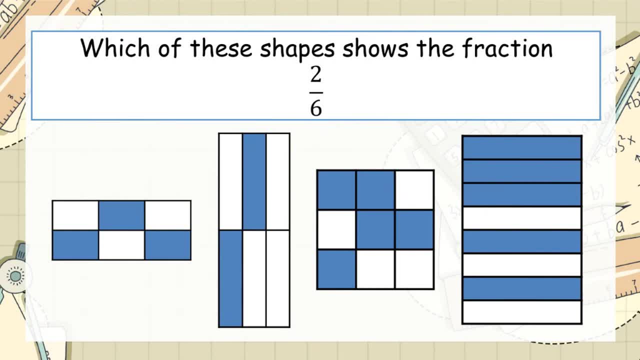 So that is going to equal to one-eighth, Which we write like this: One out of eight Great stuff. So that is our summary, So that is a fraction of a set. Take a look at these shapes down below. 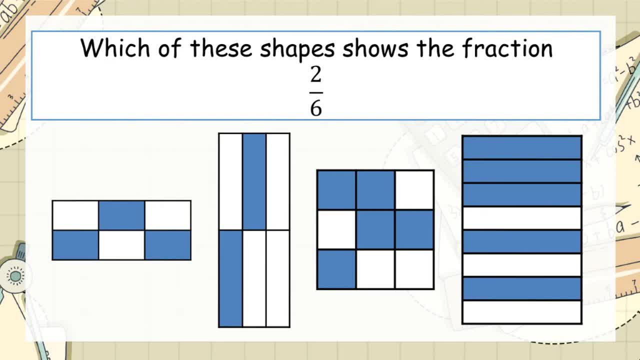 Some of the shapes have a fraction of them shaded in dark blue. One of these shapes shows the fraction two-sixths. Can you pause the video and see if you can figure out which one has got two-sixths shaded in blue? Remember, the top number of the fraction tells us how many parts are shaded. 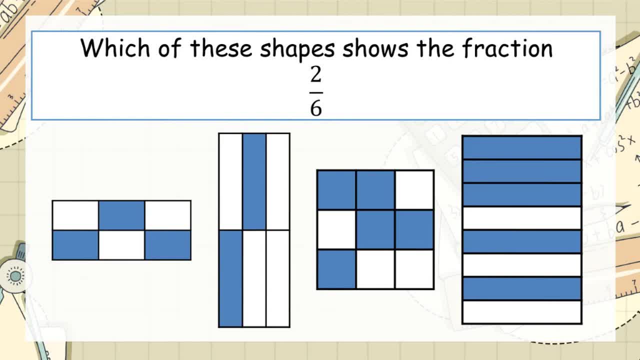 The bottom number tells us how many parts there are altogether. Pause the video and use this to help you find the correct answer. Did you get it? The correct answer is this shape here, Because you see, two parts are shaded. That is our top number. 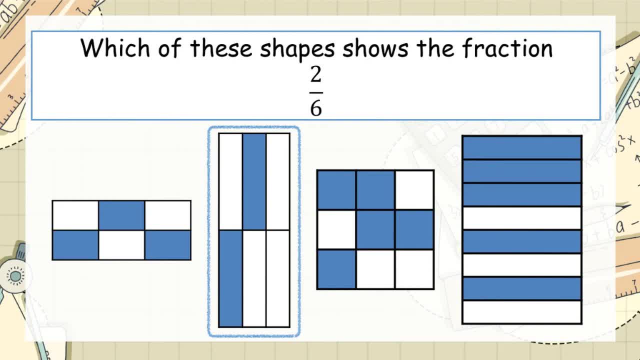 And altogether there are six parts to the shape, Our bottom number, the denominator. Here is an extra little challenge for you. Here is an extra little challenge for you. Take a look at this shape that I have marked here. We just figured out that two-sixths of this shape are shaded. 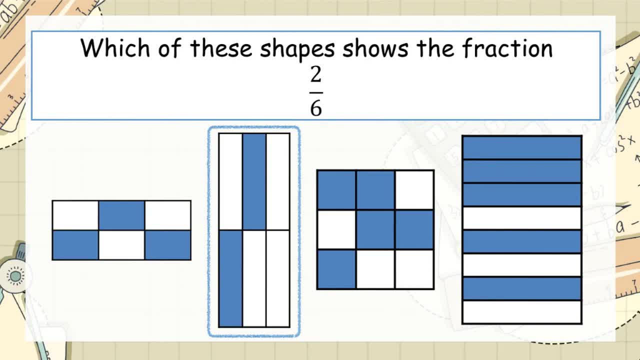 So what fraction of the shape is not shaded? Pause the video and see if you can figure that out. Well, did you get it correct? The answer, of course, is four-sixths, Four pieces out of six: One, Two, Three. 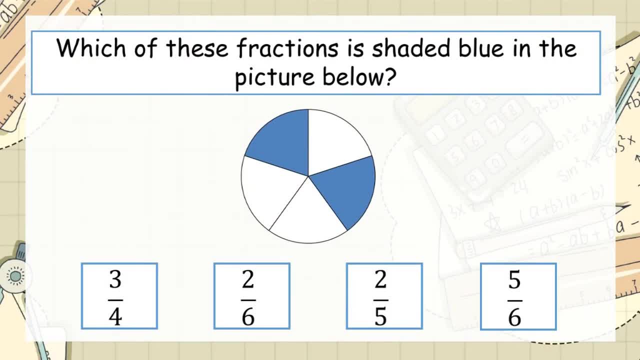 Four. Let's take a look at a different shape that's been shaded. Here we have a circle, and below there are four answers that could possibly be correct. Only one of them is right, though. Can you pause the video and see if you can figure out which of these fractions is shaded? 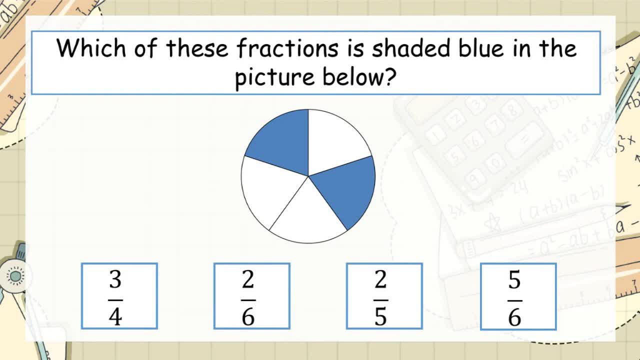 blue on the picture above. Pause the video and choose the correct answer. Remember, the top number in a fraction tells us how many shaded pieces there are. The bottom number tells us how many pieces there are all together. Use this to help you solve the question. 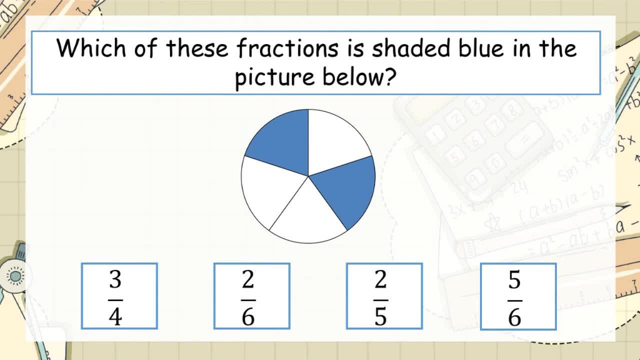 Pause the video and give it a try. So the answer we should have got is two fifths. How do we get that? Well, remember, the top number tells us how many shaded parts there are, one, two, and the bottom number tells us how many pieces there are. 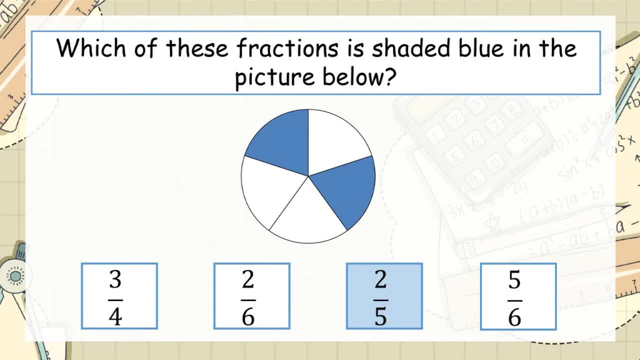 So it's two fifths or two out of five. Try that bonus question again. Now that you know what fraction of the shape is shaded, can you pause the video and figure out what fraction is not shaded? Pause the video and give it a try. 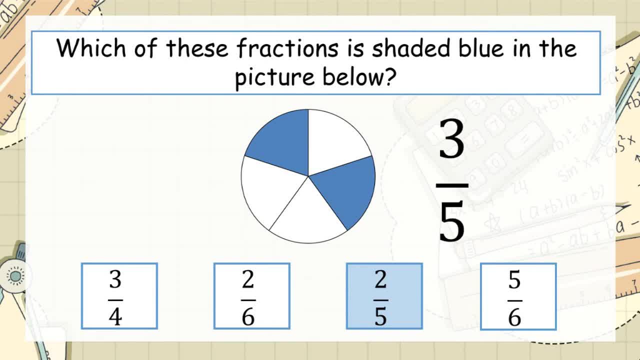 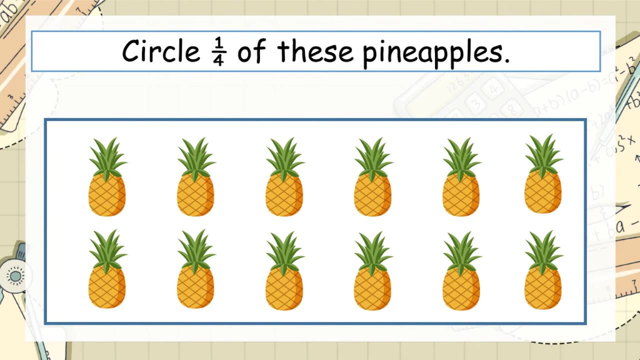 Did you get three fifths? You can see that three parts are not shaded And there's five parts all together. So our fraction is three fifths. How about if we have a question like this: We have a load of pineapples here and we want to circle one quarter of them. 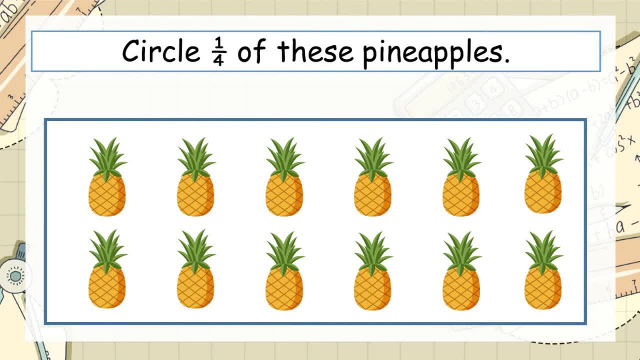 Maybe we're giving them to somebody as a gift or something. How would we find out what one quarter of all these pineapples would be? Well, this problem is a little bit trickier, because the denominator of the fraction and the total number of pineapples are not the same. 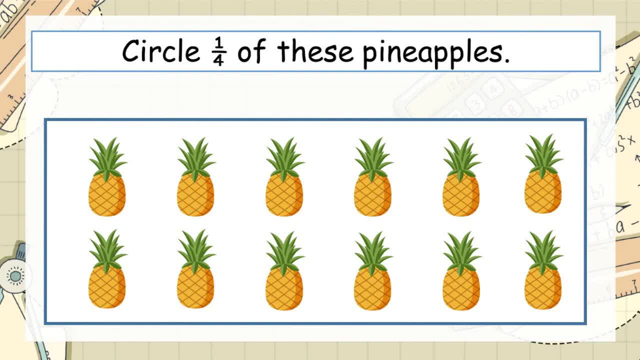 So it's not as straightforward as we're used to. First, we need to know exactly how many pineapples there are all together. So when we count them up, we're going to see that there's twelve pineapples all together. 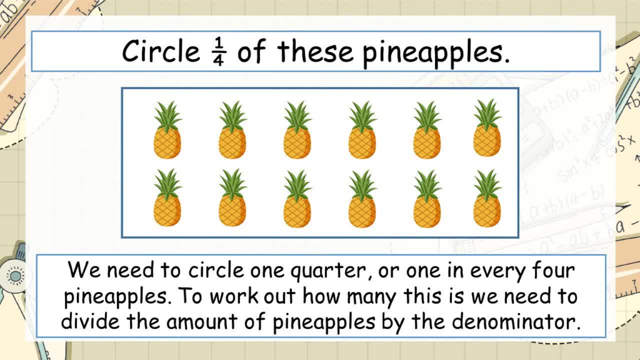 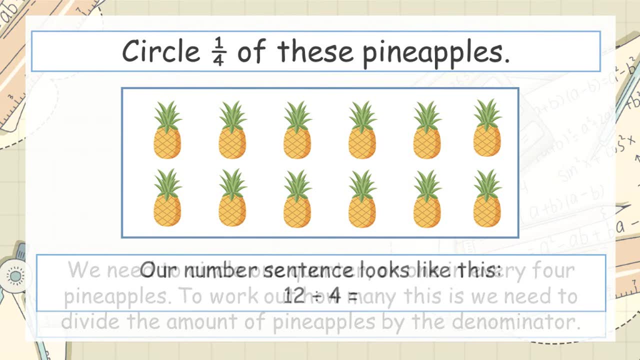 Now we need to circle one quarter or one in every four pineapples. To work out how many this is, we're going to need to divide the total amount of pineapples by the denominator of our fraction. Our number sentence would look like this: 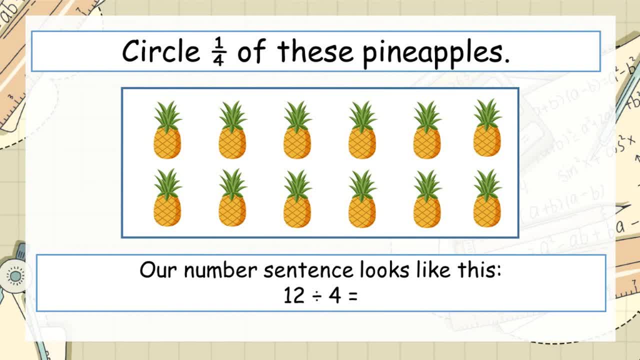 Twelve divided by four, And when we divide twelve by four, the answer is three. So we needed to circle three pineapples to show one quarter of the set. Now, using division is definitely the best way of finding fractions of bigger numbers, But for now we're going to use division. 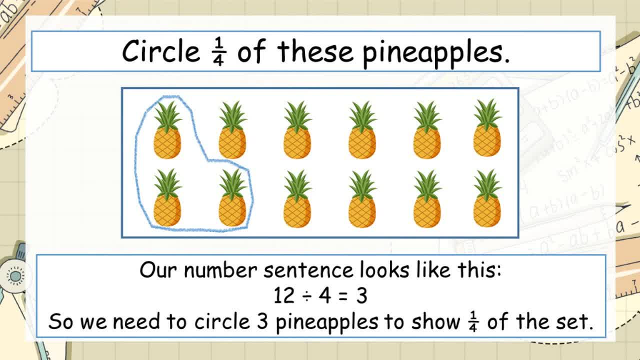 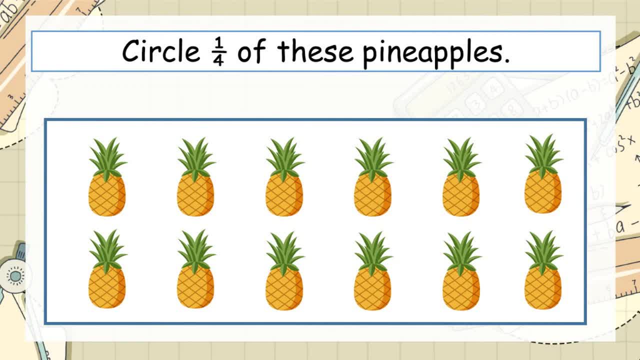 We want to find out what one quarter of these pineapples are, Because we understand that the fraction one quarter means one out of every four pineapples. what we can do is circle every fourth pineapple: One, two, three and circle the fourth. 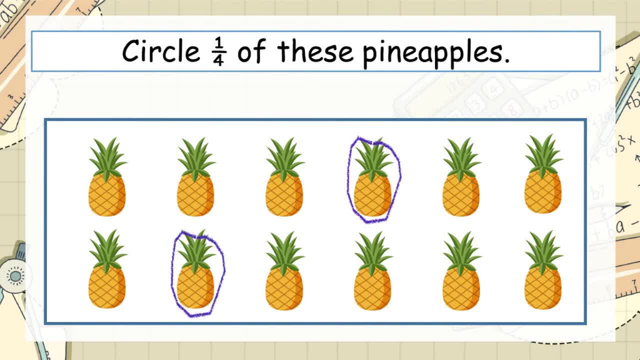 One, two, Three And circle the fourth. One, two, Three And circle the fourth. You see we got the same answer: Three pineapples are circled. That's because we circled one out of every four pineapples. 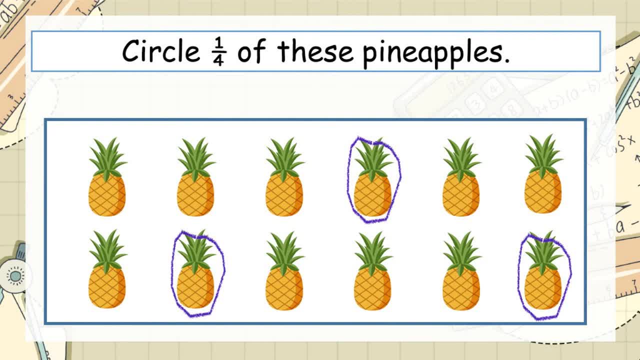 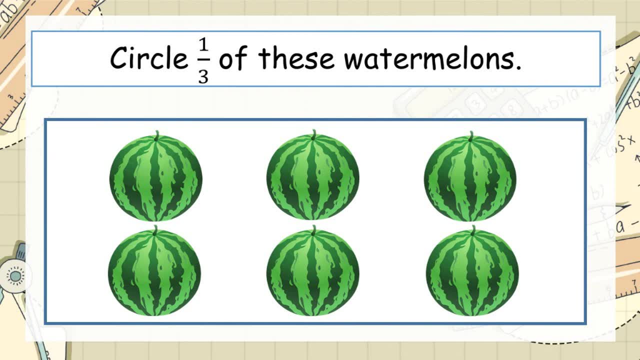 Or one quarter of the pineapples. Using what you just learned, try and circle 1 third of these watermelons. Either use the division way or do the counting way. Either use the division way Or do the counting way. 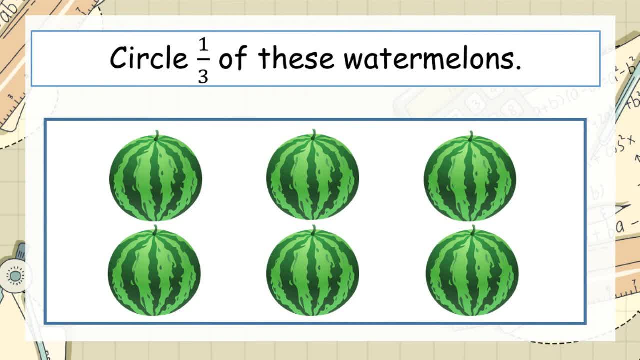 Either do the division way Or do the counting way, It doesn't matter, You'll get the same answer. Pause the video and give it a try. Well, how did you get on? Remember, we need to circle one third or one in every three watermelons. 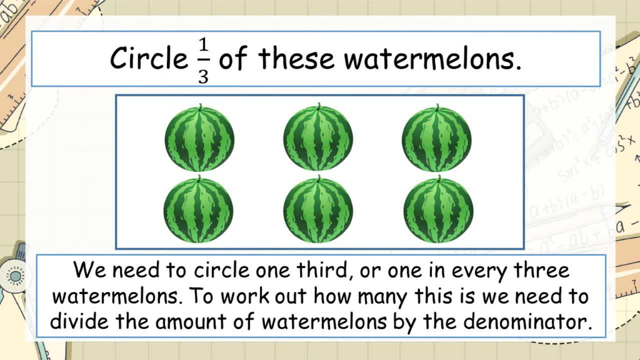 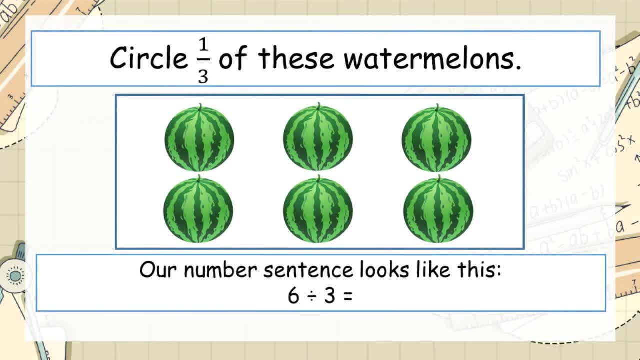 To figure out how we might do this, we can divide the amount of watermelons by the denominator. In this case that's three. So six watermelons divided by three is equal to two watermelons, So one third is equal to two. 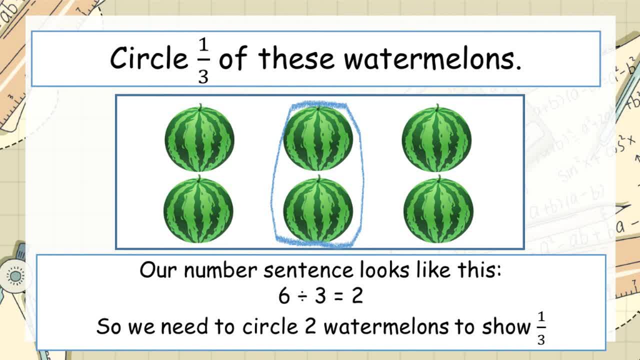 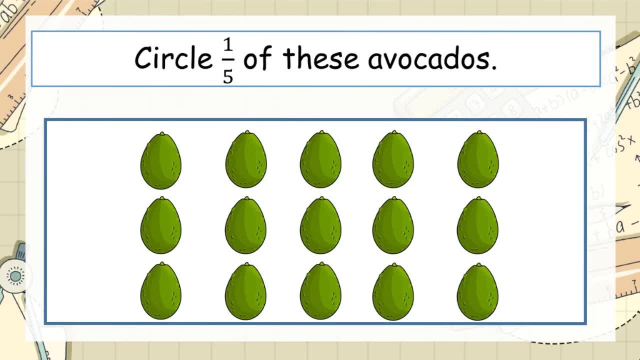 You would get exactly the same answer if you marked one in every three watermelons. See, Okay, try this one all by yourself. I want you to circle one fifth of this group of avocados. Either divide the total number of avocados by the denominator and find it out that way. 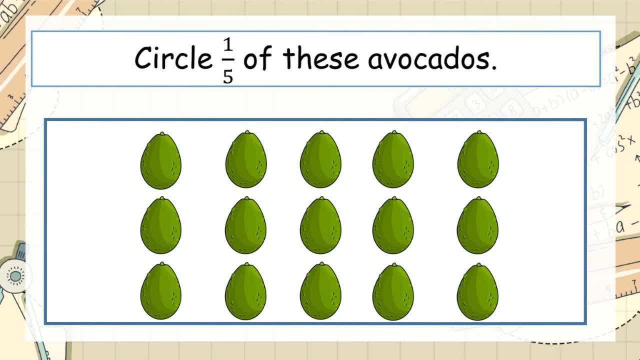 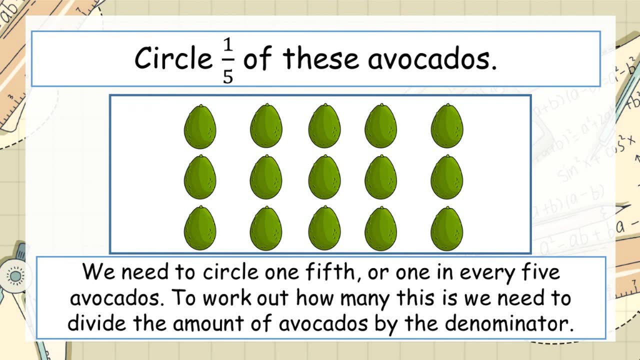 or circle one in five avocados. Pause the video and give it a try. Well, how did you get on? So in this one we needed to circle one in every five, or one fifth of all the avocados. 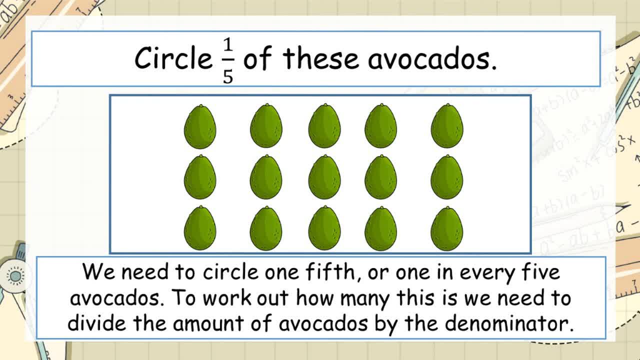 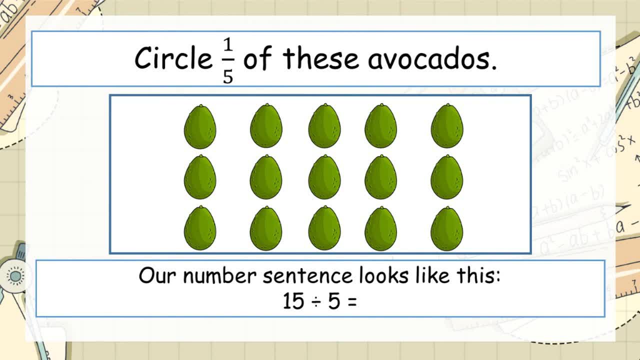 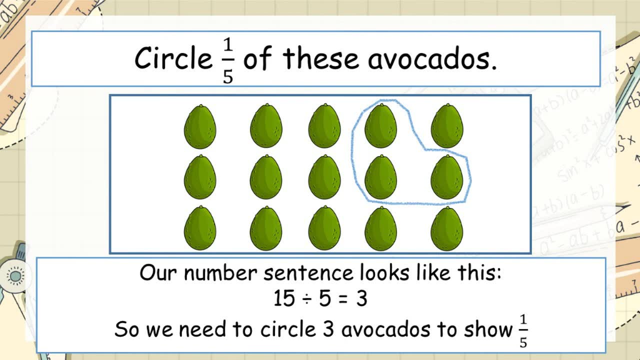 To work out how many this is, we divided the amount of avocados by the denominator, And that gave us this number, sentence fifteen divided by five, And our answer is three. You needed to circle three avocados to show one fifth.